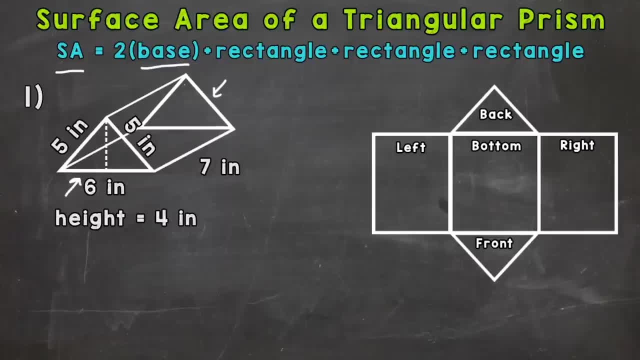 exact same size and shape, So we only need to find the area of one. That means we have the area of both. So we'll start with. area equals one-half base times height. That's the formula for the area of a triangle. So let's plug in now. So one-half times the base is six here. So six that's six. So we're going to. 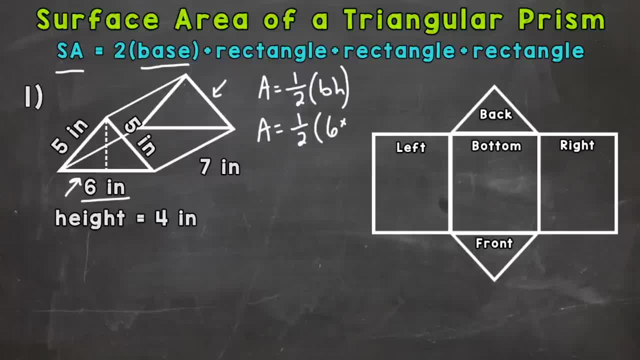 times the height, which is that dashed line, and the height is 4 inches. so let's solve: 6 times 4 is 24 times 1, half is 12. so we have 12 square inches there and we multiply that by 2 again, because we have two bases and they are the exact same. 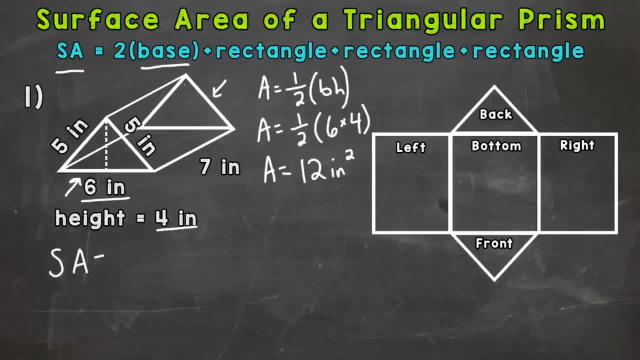 size and shape. so let's write everything out down here below the problem. so surface area equals and we will plug in our first area, 12 square inches. and now we get to the rectangles. but before we start that, I want to take a look at the right-hand side of your screen and we have our triangular prism unfolded, that's. 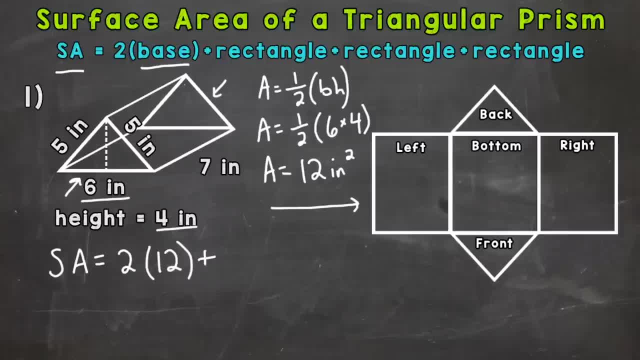 called a net, so everything's unfolded. it's going to give us a better idea of the areas of the faces and it helps us visualize what we're doing here when we unfold the prism. so let's take a look at the right-hand side of your screen and 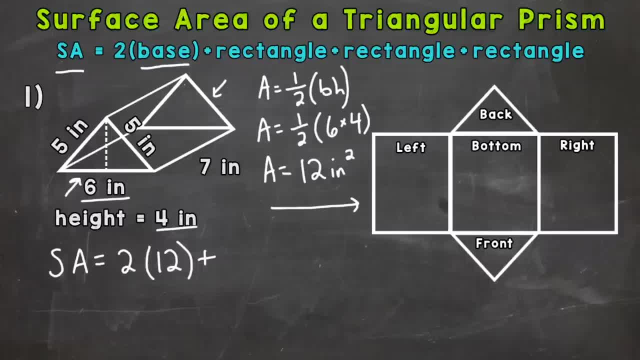 fold that 3d shape. so try to visualize unfolding it or even folding that net back up and creating the 3d triangular prism. so let's get into the rectangles. so we have a bottom rectangle, a left rectangle and a right rectangle. now the left and right rectangle are the exact same size. the bottom one is different. so 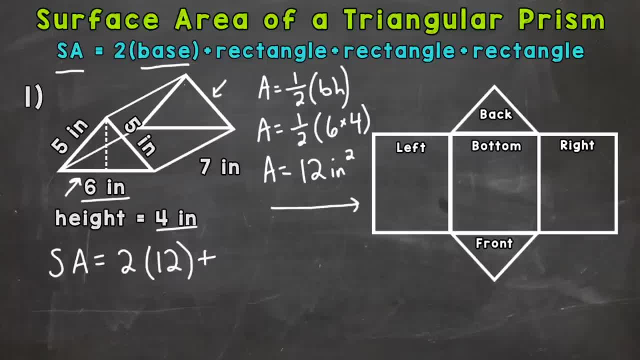 let's do the bottom rectangle first, so we can think of this as the bottom rectangle, and then the bottom rectangle, and then the left rectangle, and then the rectangle here, the right and the left, it doesn't matter what order you do them in. you'll get the same answer either way. but we're starting with the bottom, so 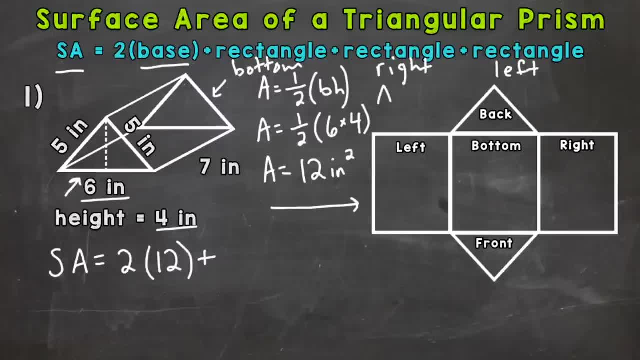 let me fill in. trying to find some room here. we'll do. area equals length times width. so length times width for the area of a rectangle. you can also use base times height, so whatever works best for you. so let's plug in. area equals. well, the length is. 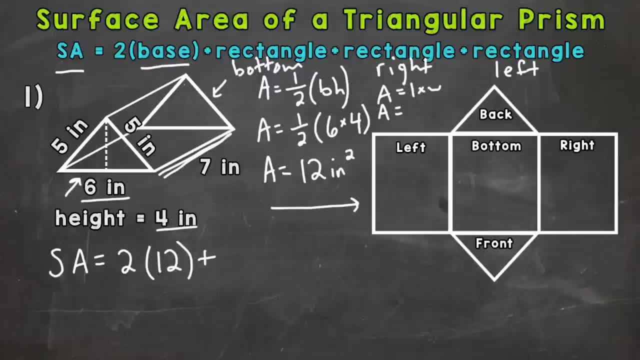 seven inches here and the width is six inches. so we have a seven by six rectangle or six by seven. either way it will give you the same answer. so seven times six and our area equals forty-two square inches for that bottom rectangle. so we'll plug in here 44 and let's actually write on our net here: this is: 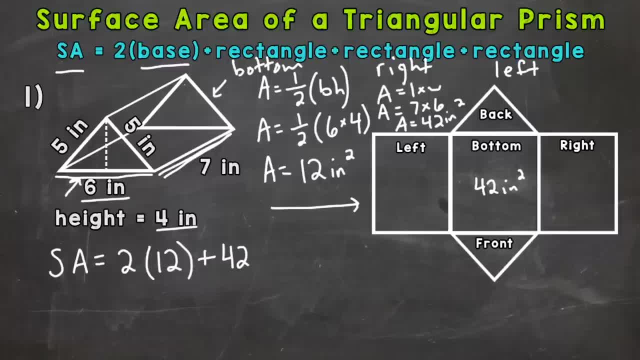 going to be 42 square inches. the front triangle, remember, is keeping that table value Linear with the 60, and this is the new конечно example. really that's going to・・・ remember- is 12 square inches and the back triangle is the same. so let's do. 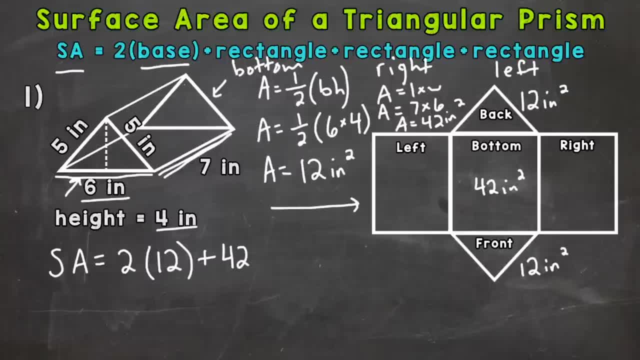 the right and left, and these rectangles are the exact same, so we only need to write out one here. so let's go to the bottom of the screen. area equals length, times width- and let's plug in, so we have a length of 7 and a width of 5 here. so 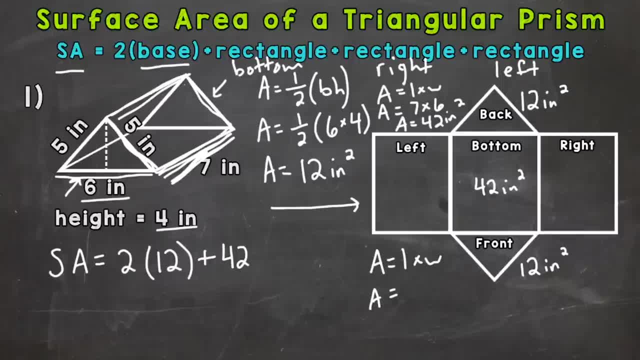 if you're having trouble picturing the rectangle, it's this right rectangle here. so 7 times 5, or if you did 5 times 7, you'll get the same answer either way. so area equals 35 square inches, so 35 and again, this is the right one we did. but 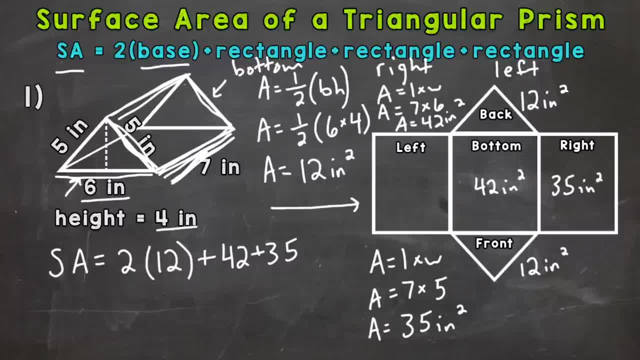 the left one is the exact same in the case of this triangular prism. so 35 square inches. so let's add another 35. and now we are good to go as far as adding this up. so we get 2 times 12 is 24 plus 42 is 66. and then we have 35 plus 35, which is 70. so 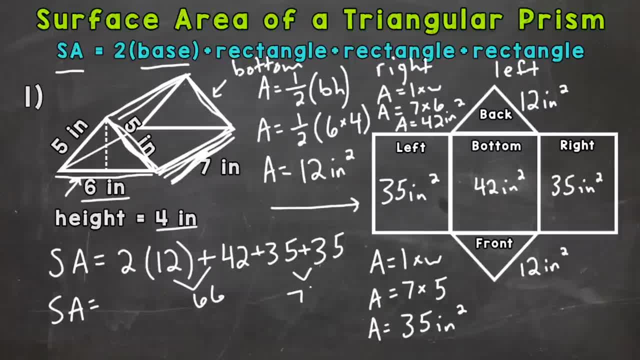 this is 66 here, this is 70. add those together and we get 136. so surface area equals 136 and that is square inches. now that was a lot of work there as we went through. now, the more of these problems you do, the better you'll get and the quicker. 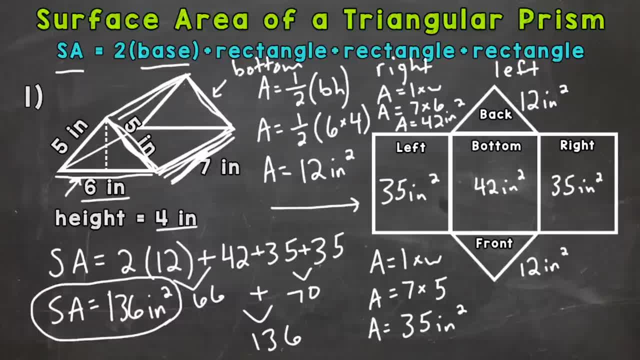 they'll go. I kind of laid everything out and went slowly as to really explain each step, but again, the more you do, the quicker and better you'll get at these. so just to recap, when it comes to finding surface area, find the area of each face and then add another section of the.